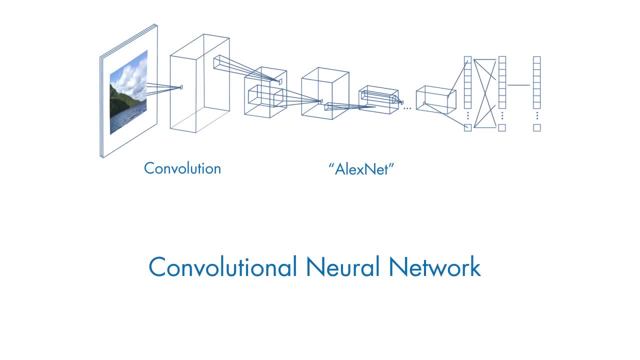 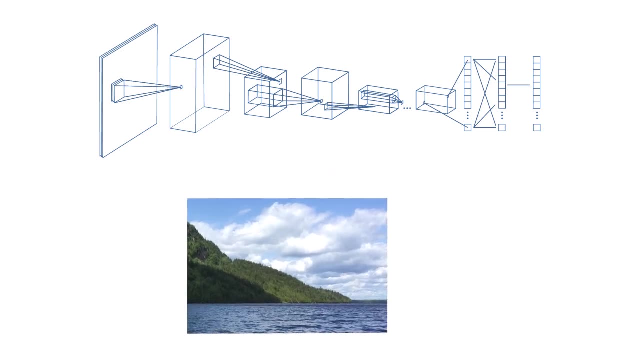 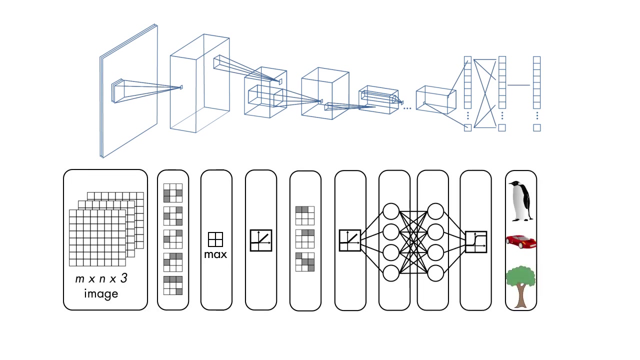 The pre-trained networked. AlexNet is an example of a convolutional neural network, or CNN. CNNs are a powerful, commonly used type of neural network designed for applications where the input has an inherent two-dimensional structure like an image. Like all neural networks, CNNs are made of layers and information is passed between those layers. 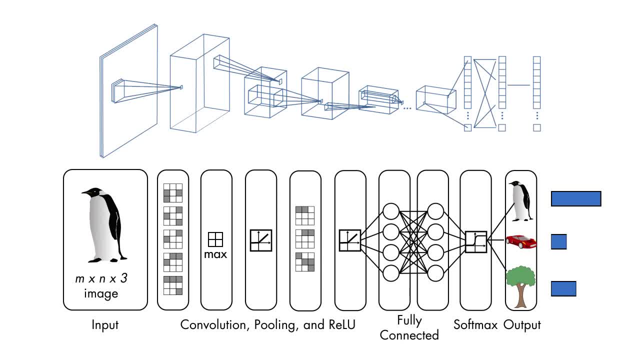 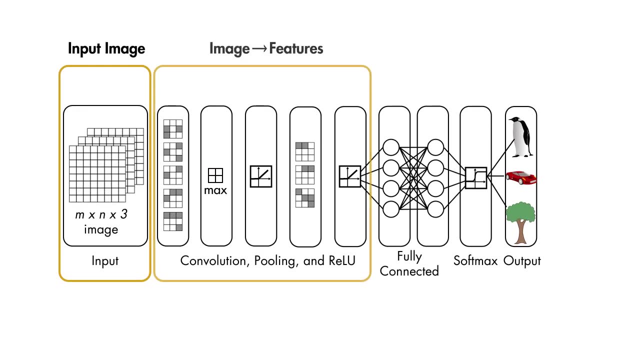 For a classification problem like this one, the output layer returns the strength of the network's prediction for each possible class—penguin, car or tree. There's a lot more detail to the various kinds of CNN layers, but broadly speaking, the bulk of the network turns the input image into a set of features that the last few layers then use to perform the classification. 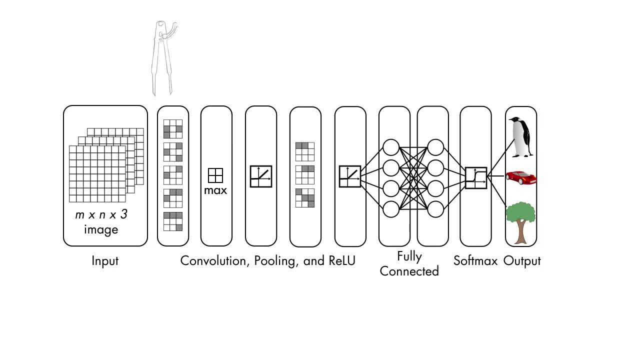